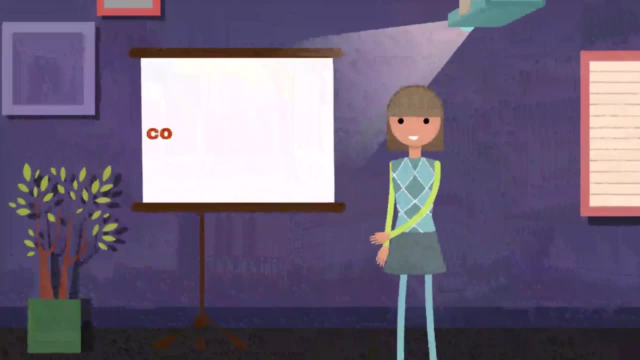 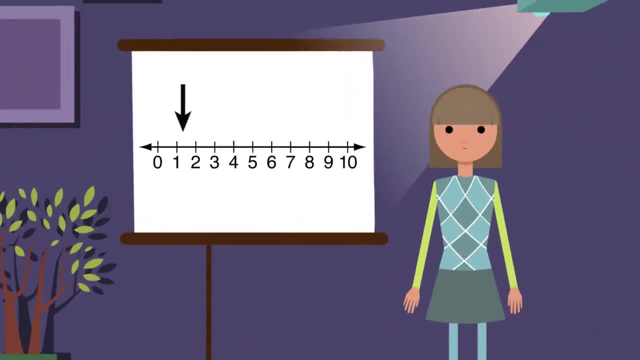 We can use number lines to compare numbers. Let's compare the numbers 4 and 8.. First start with 0 and count up to 4 with me. Ready, 1, 2, 3, 4, Perfection. Now count to 8 with me. 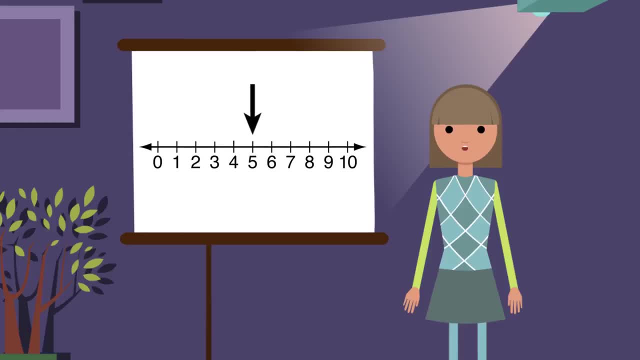 1, 2, 3, 4, 5, 6, 7, 8. Great. Now compare the lengths of the lines. Which is bigger? You got it. The line from 0 to 8 is longer than the line from 0 to 4. This shows that 8 is bigger, or worth more than 4.. 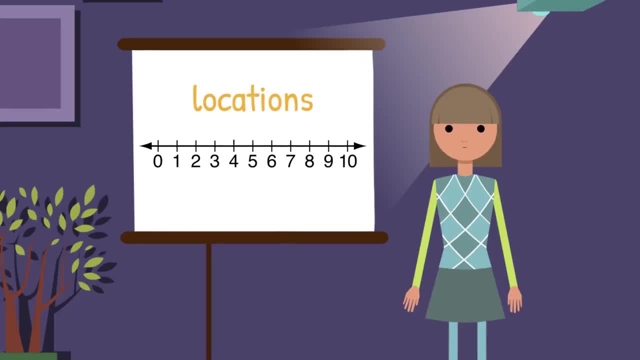 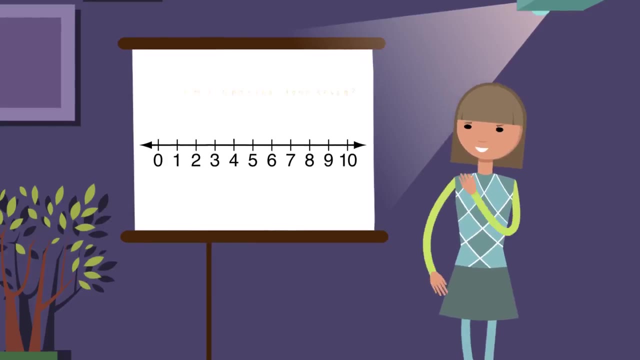 Now let's take a look at another number line, a closer look at locations on the number line. find the number seven. we can see eight comes after seven on the number line. so eight is larger than seven. this number line counts up by ones. so eight is one more than seven. what is one less than seven? 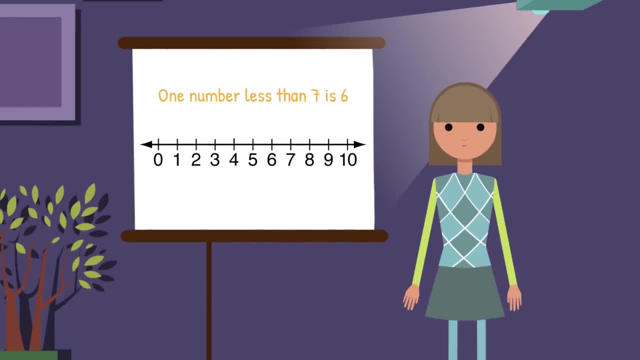 you are so smart. one number less than seven is six. since it is one place behind the seven on the number line, six is one less. we can say six is smaller than seven by one. let's look at another piece of the number line with bigger numbers. if we continued counting down this number line by ones, 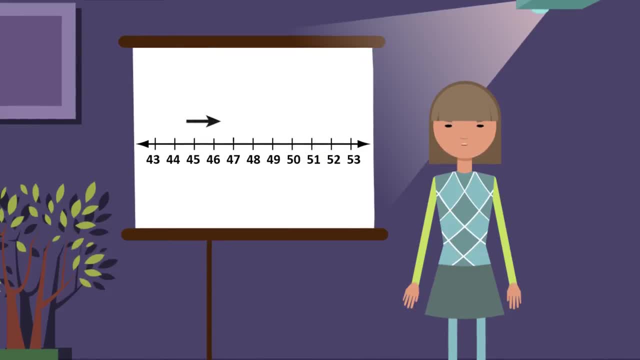 we would reach this section. number lines can go on and on, just like we can count on and on. bigger numbers work, just like the smaller numbers on a number line. some number lines may count up by twos or fives, but this number line counts up by ones. are you ready for a? 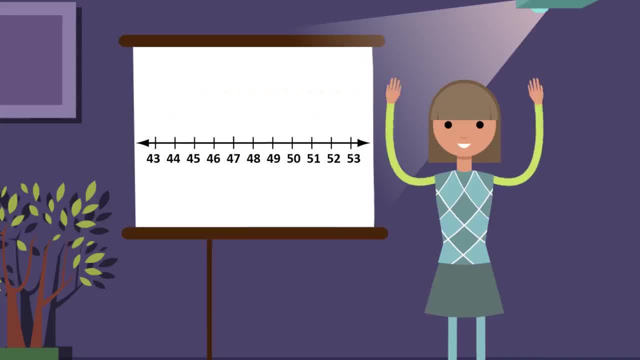 quiz. okay, use the number line and say your answer out loud. what is one more than 44? 45 is correct now. what is one less than 51? yes, 50 is correct. what is one less than 50.. 49 is spot on. that was awesome. you definitely know how to use a number.